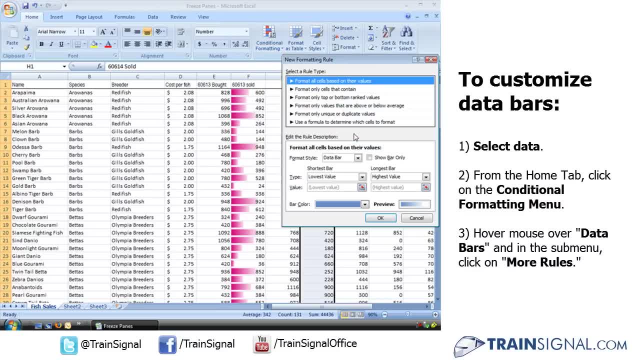 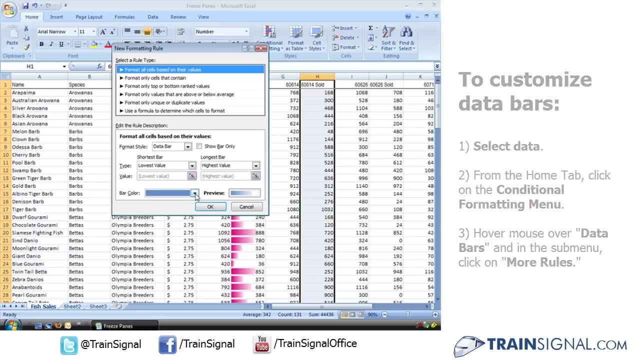 formatting data bars. Let's take a look at more rules and see what else we can do. We can go ahead and select first of all a different color, But let's not worry about that right now. We're going to go ahead and the type is lowest value. What if we want to? 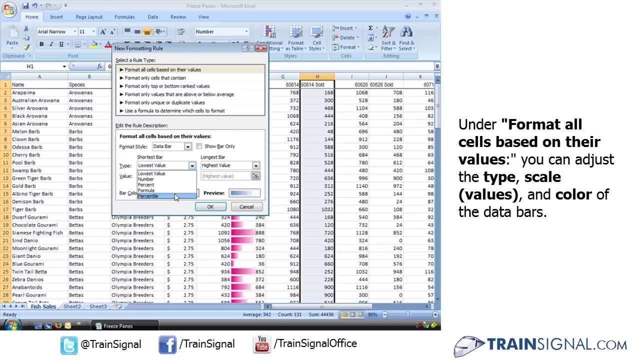 choose number, percent formula, percentile, things like that. Now, of course we don't have percentages. actually, it will be the same if I choose number and pick a value. let's say 0 to 1500. and let's pick a color. how about purple? that will be nice. 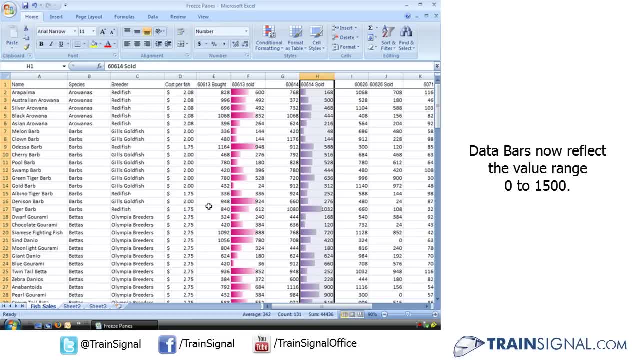 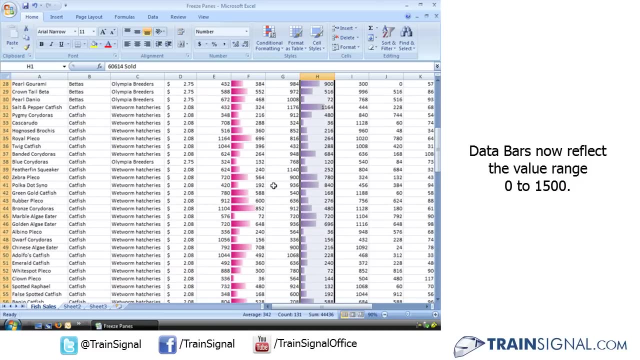 and now it shows us those data bars. relative to that range, we set 0 to 1500. see the difference between this 1032 and say this 1032, because this one is basing the top on 1500, this one is taking the highest value. 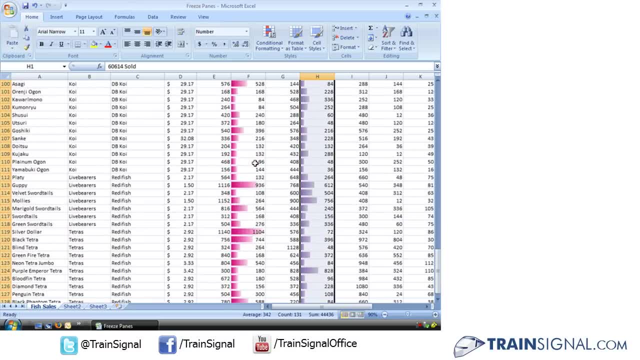 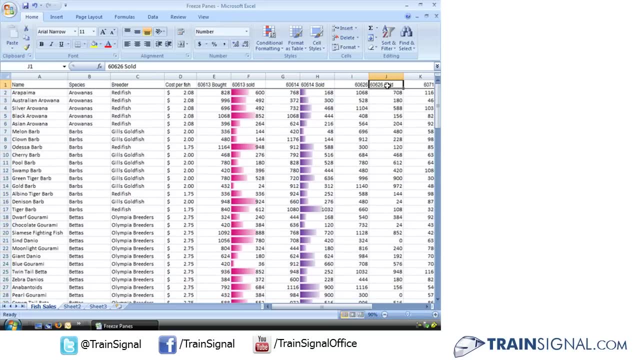 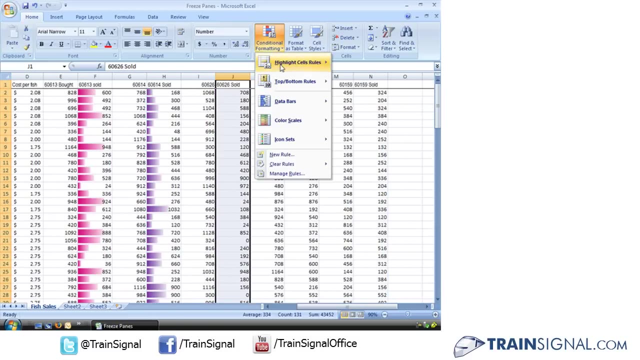 which I believe is 1032 in here- nope, it's 1104- and making that the top value. alright, let's go ahead and let's move down a little bit further and let's select some more data and we'll go, instead of our data bars, to color scales. 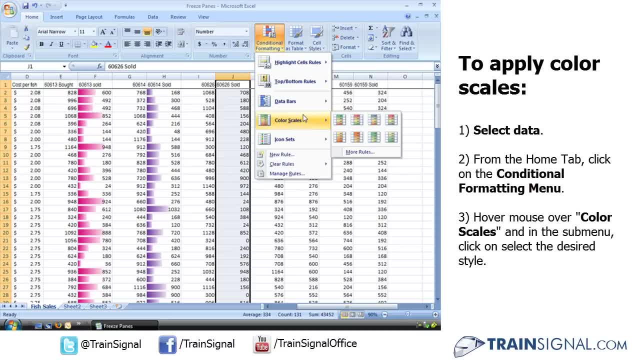 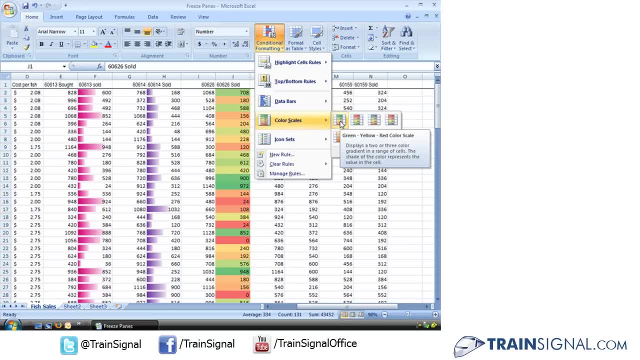 now color scales. basically the same thing, but instead of data bars it uses a range of colors. now let's take a look at this one here: green, yellow, red color scale displays a 2 or 3 color gradient in a range of cells. 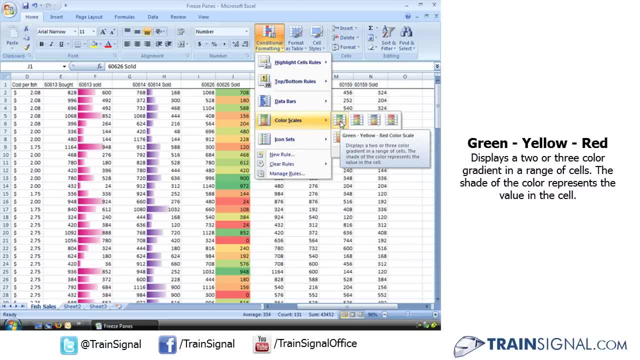 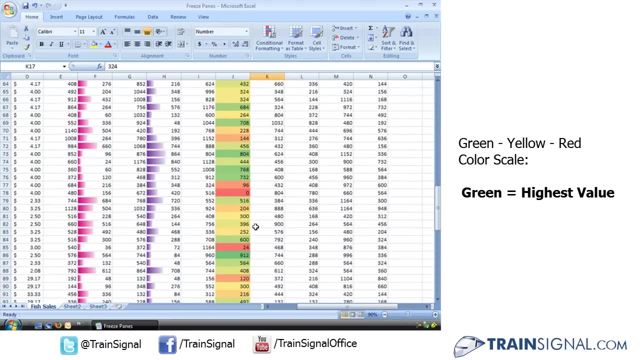 the shade of the color represents the value in the cell. now, when we look here, we see that the green is on top and the red is at the bottom. that means the green is going to be the highest values and when I click on that you can see exactly that. if I go ahead and I look, 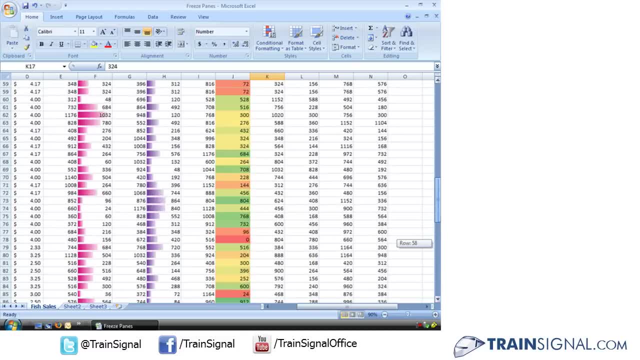 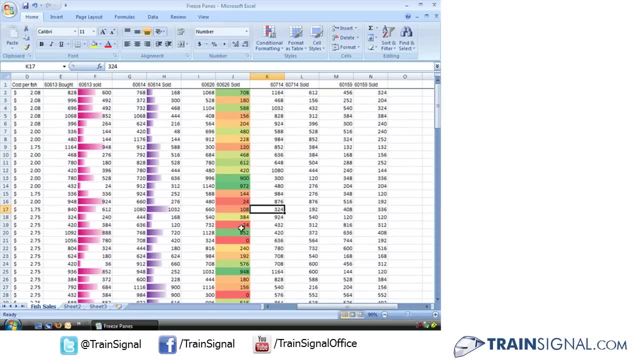 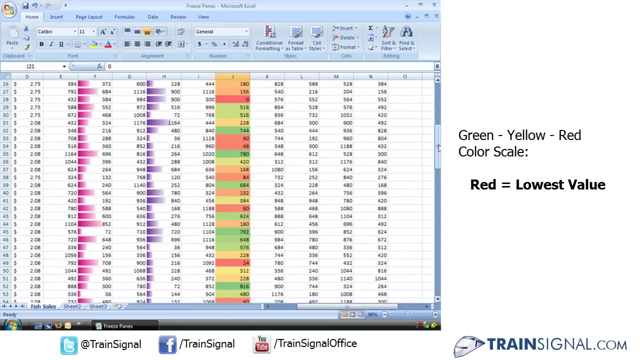 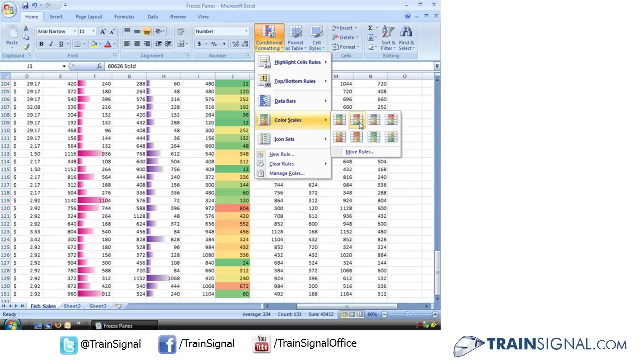 through here. see, like 900, is that dark green? 948 down to, through that color range, the lowest. well, there's a zero, which is that dark red. I can also go ahead. let's take a look here and change it so that the red is the highest value, and watch as I change these.